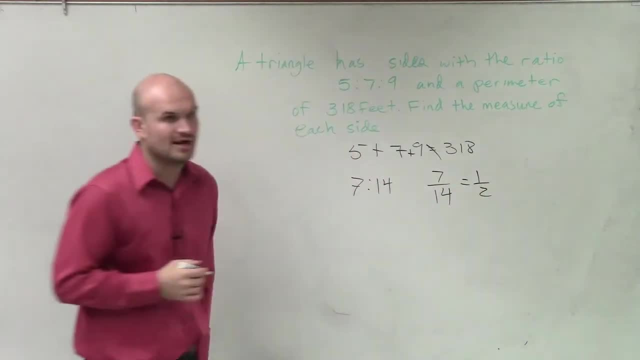 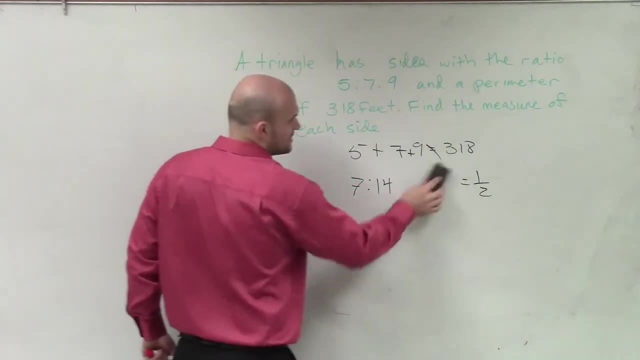 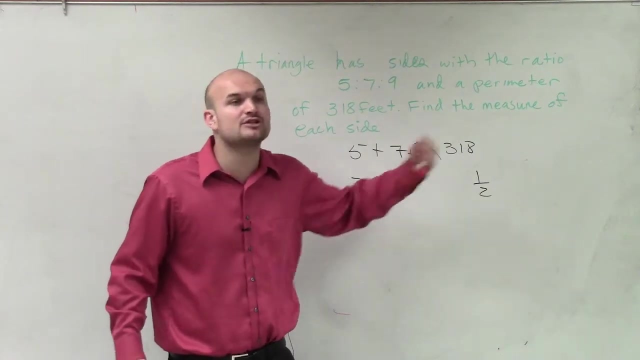 the ratio. So we would write that as one half right For every girl. there's two boys in this classroom. But if you just look at this ratio and forget about the 7 over 14, is there one girl and two boys in this class? No, there's 7 over 14, right, But we reduced the ratio. 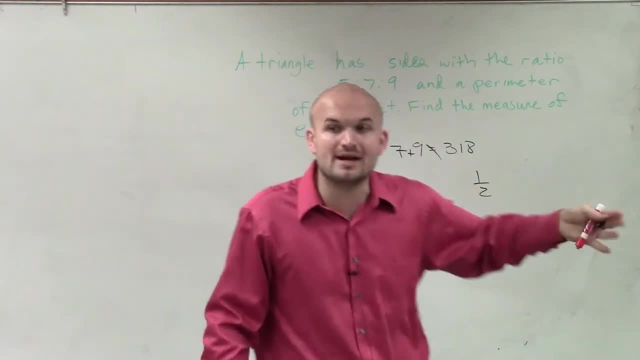 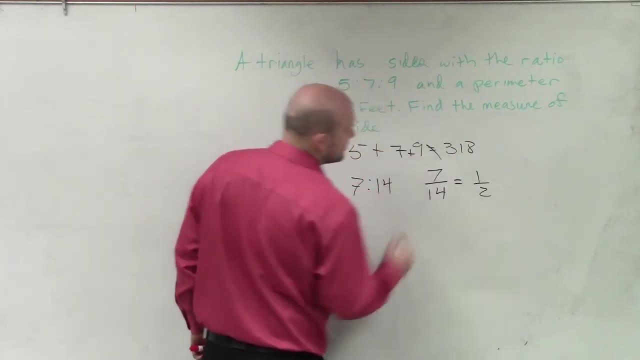 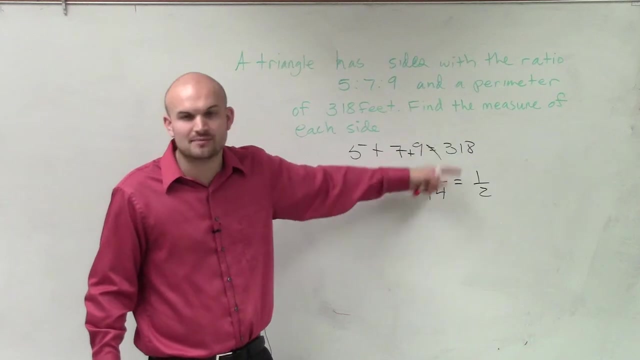 We reduced extended ratio, But what we want to do is find well, what then, exactly are the exact side lengths? So, to get to 7 over 14, right, I divided by a number on the top and bottom, And what did I divide by? What did I divide by on the top and bottom to get? 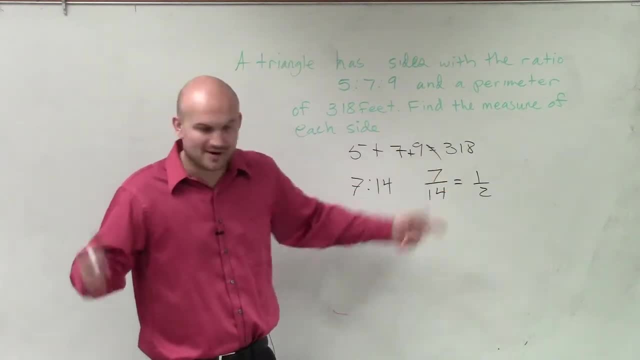 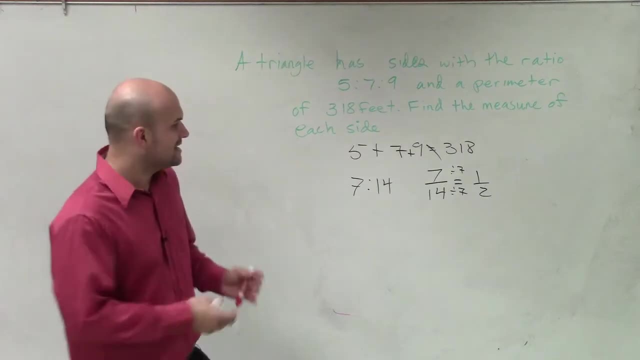 one half 7.. But give me 7, right, That's okay. So I divided by 7, right. So what I'm pretty much asking you guys is if this is already reduced. So if I divided 7 to get to one half, I would have to multiply by 7 from one half to get. 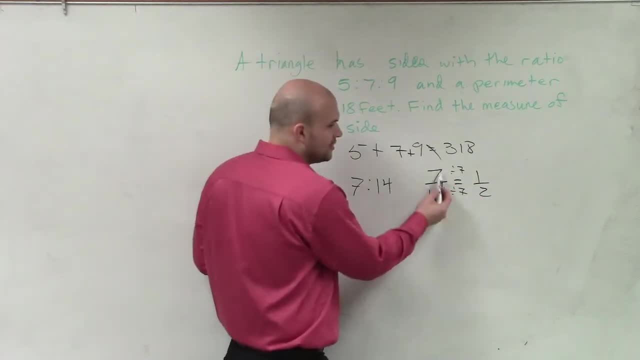 to 7 over 14, right To go from 7 over 14,. I'm dividing by one half to get to one half. I'm dividing by 7 to get to one half. correct, If I had one half and I say what was actually. 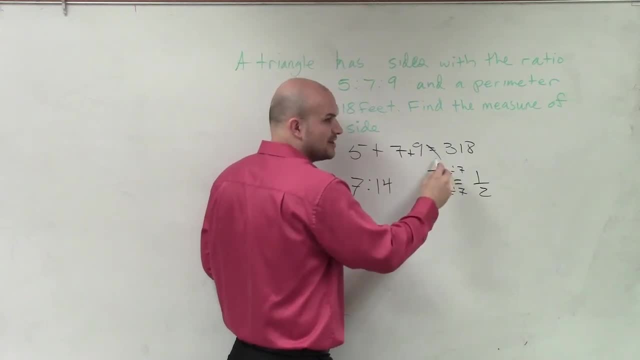 the number in this classroom, I would have to multiply. I'm just doing the reverse operation To go from here: I divide. If I wanted to go back I would have to multiply, correct. So I'd multiply with 7.. 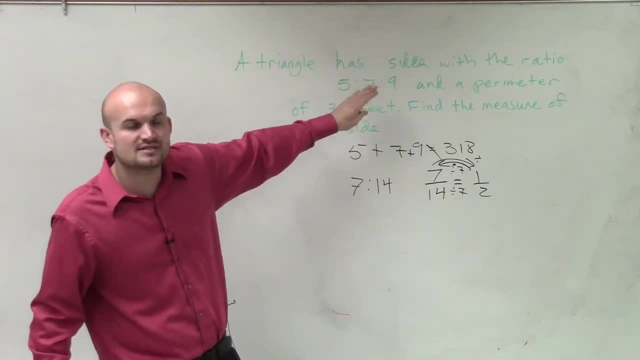 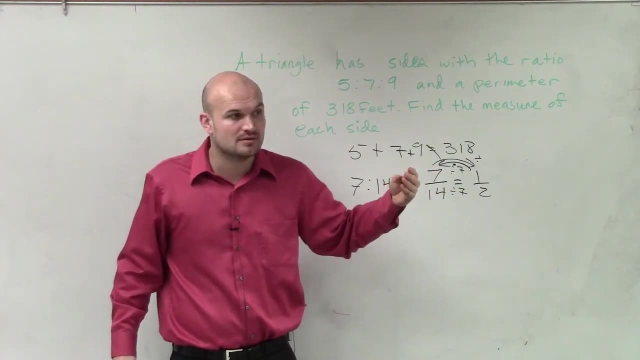 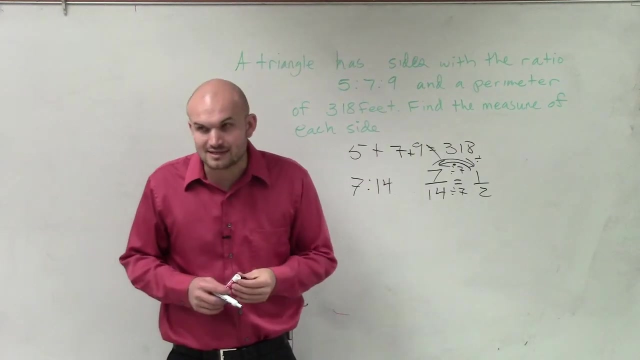 And this is a reduced rate or a simplified extended ratio. So what I need to do is I need to multiply it by a number. I need to multiply it by a number to get to my exact side lengths. Do we know what that number is? No, This one we know, because we had two. 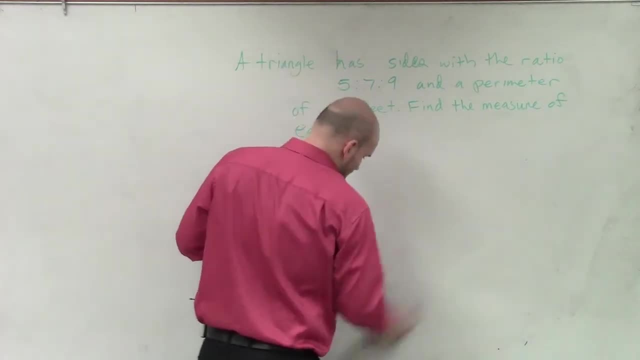 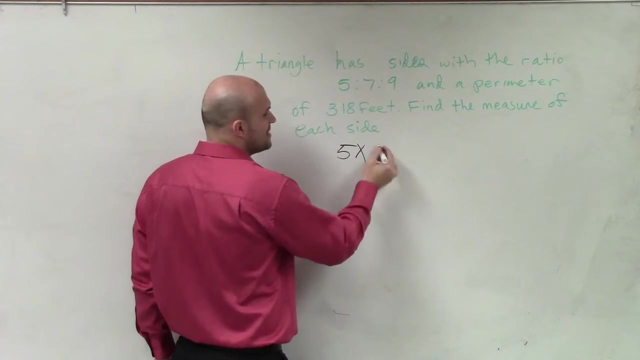 numbers, but we don't know what that number is. So I know that 5 times a number. well, if we don't have a number, we don't know what that number is. So we're going to multiply it by a number. Let's call that x, 5 times a number, plus 7 times a number plus 9 times. 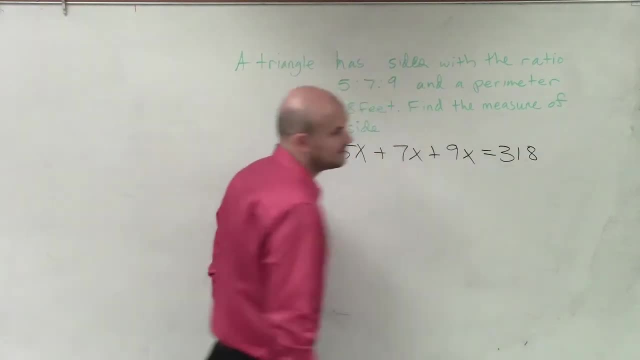 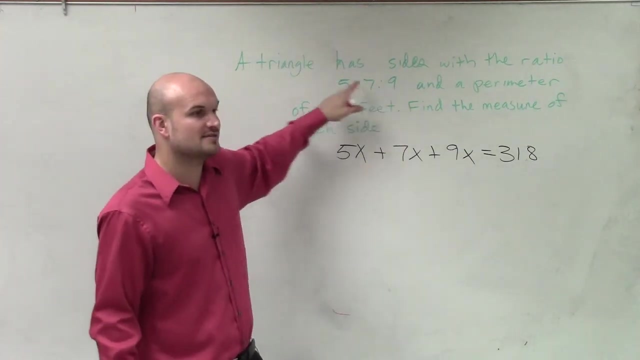 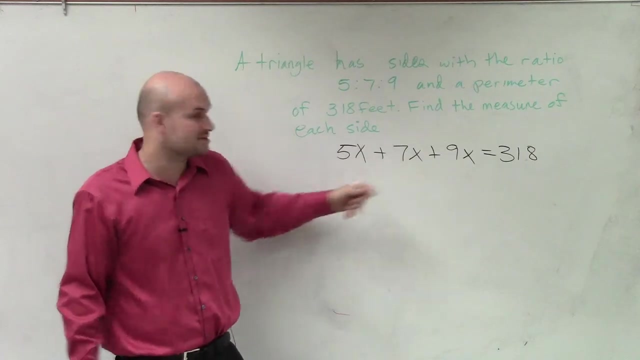 that same number equals 318.. So that's how you would go ahead and set this problem up. These are not the lengths of your sides. We're trying to find the lengths of our sides, but this is reduced, So we need to multiply it by a factor to get our correct numbers. So therefore, I have 5x plus 7x plus.